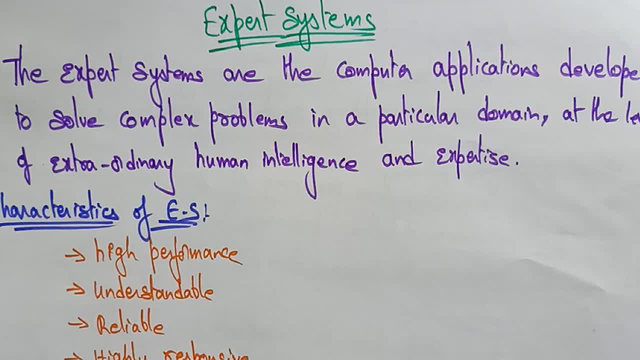 Hi students, welcome back. Let's continue with the scope of artificial intelligence. So far you have seen about the game planning and the natural language processor. Now, coming to the another scope of this artificial intelligence is the expert systems. The expert systems or the 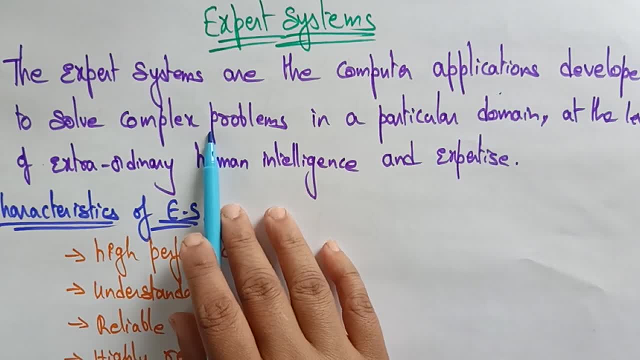 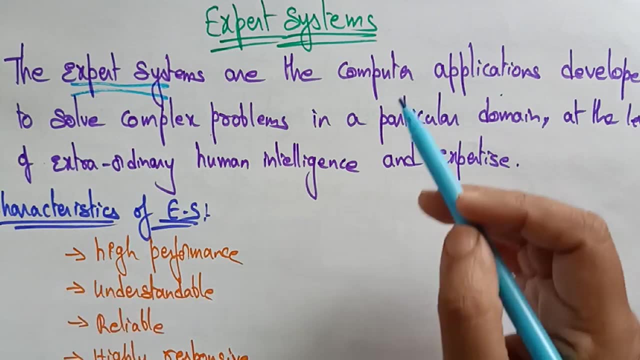 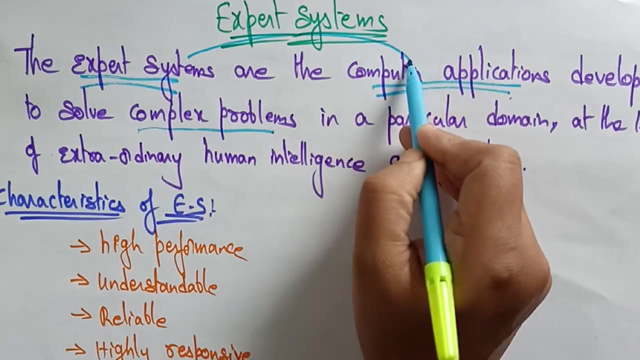 computer application developed to solve the complex problems. So we are here, we are using some expert systems. What is the use of these expert systems? It was the expert systems or the computer applications developed to solve the complex problems. So it means the expert system. 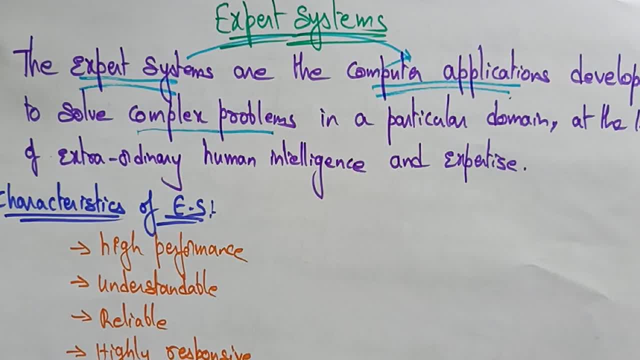 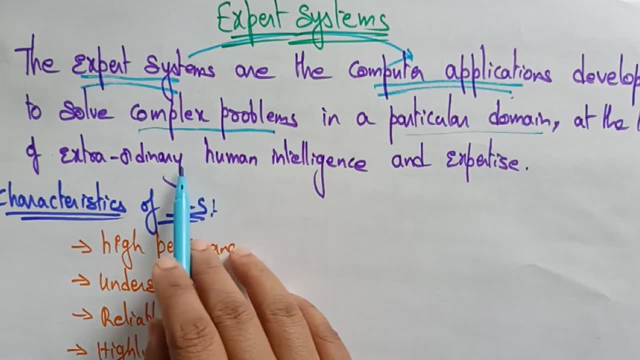 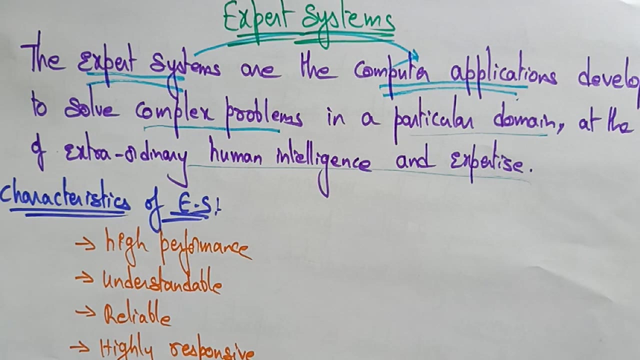 is nothing, but it is a computer application for solving the problems in a particular domain at the level of extraordinary human intelligence and expertise. Okay, so the expert- the name itself is saying it is an expert system and it is one of the computer applications which is used to solve the. 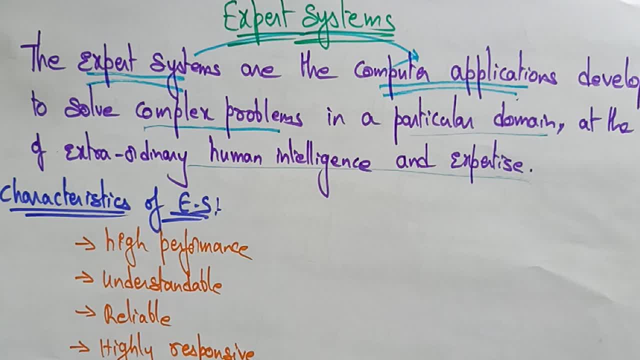 complex, complex problems In a particular domain. whatever the domain you are taking, either you are taking the car- it's automatic car you are taking, or your self-driving car you are taking, or any game playing you are taking. whatever the complex problem you are taking at that particular domain, 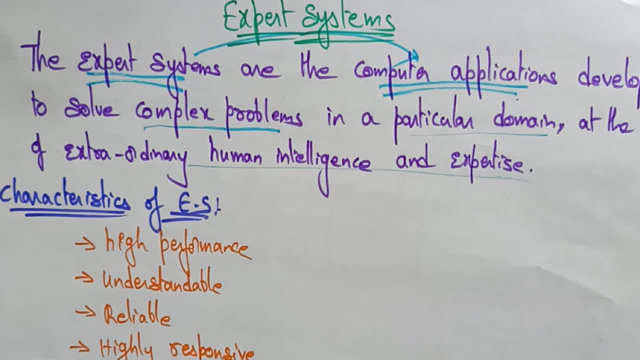 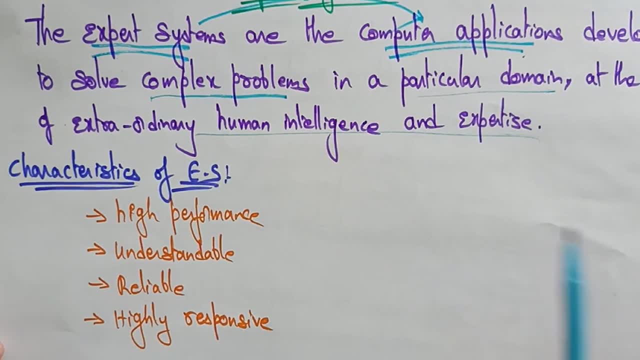 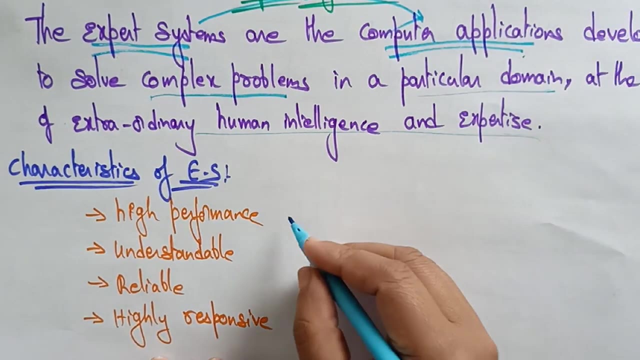 it is a level of extraordinary human intelligence and expertise. Okay, let's see the characteristics of the expert system. The characteristics of this uh uh uh application, computer application, that is expert system- is it's a high performance. the expert systems are high performance, understandable, reliable and highly responsive. okay, so these are. 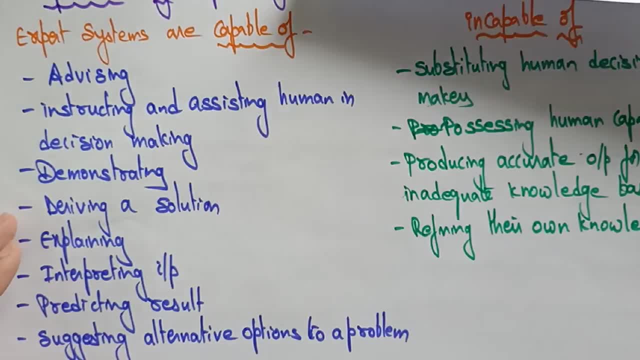 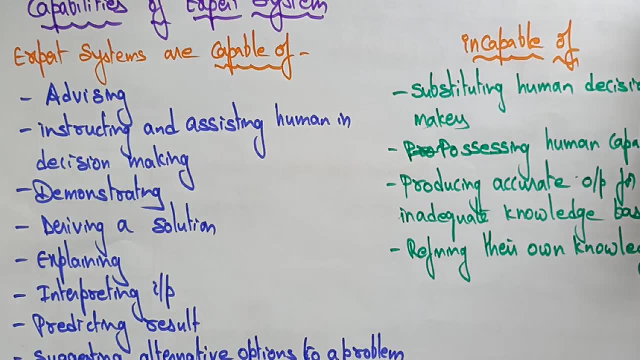 all the characteristics of the expert system. now let's see the capabilities of expert system. i'm saying that expert system is just an extraordinary human intelligence and expertise which is one of the computer applications for solving the complex problems in a particular domain. so what are the capabilities and incapabilities of this expert system? let's see the capabilities of the expert. 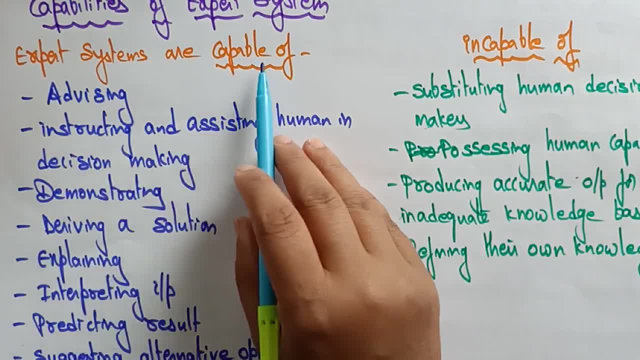 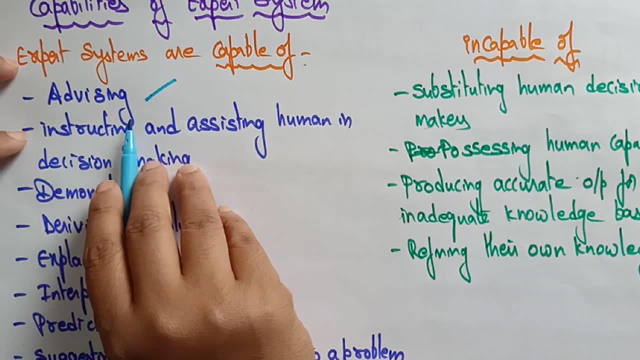 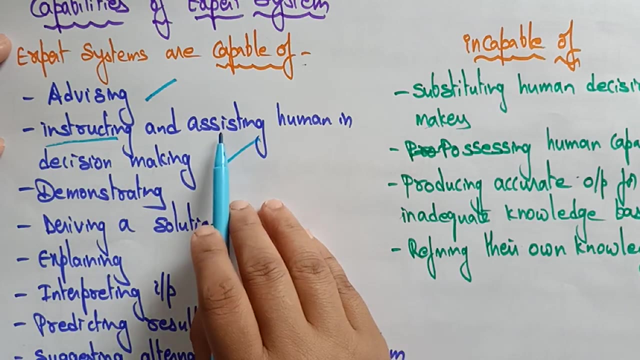 system capable and in next, incapable. the expert systems are capable of advising. okay, it is advising to everyone, giving advices to the everyone, instructing and assisting human in decision making. so it is also helping in instructing you, assisting human in decision making, what the expert systems in the artificial intelligence. 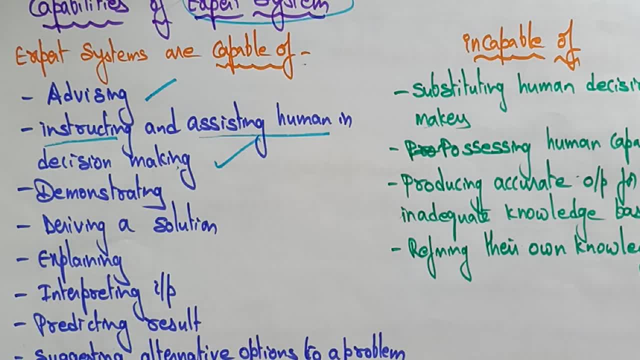 it is going to instructing you and it is assisting you- uh, human- in decision making. next, demonstrating. so, whatever the question you are asking, it is giving the response. okay, based on the input, uh answer given by some other. okay, it's just giving answer to this, demonstrating to you deriving a solution. so, whatever the question you are given based on, 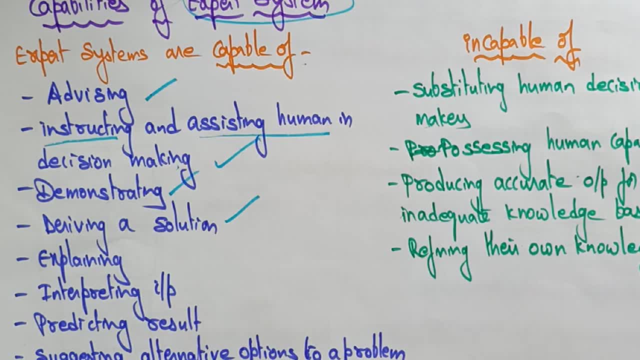 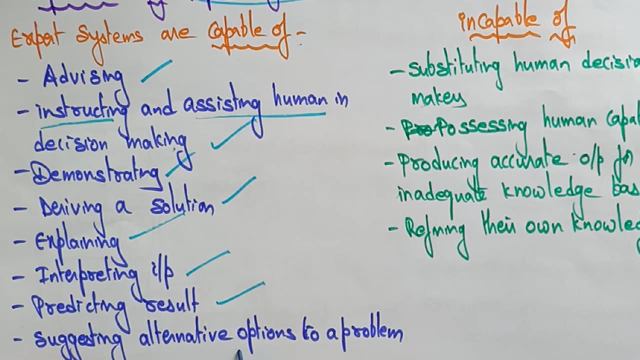 the knowledge that it is having, what, based on the knowledge that the experts uh has uh integrated in it, it is going to solve the solutions also for the problems: explaining, interpreting input, predicting result and suggesting the alternative options to a problem. so it is also going to suggest the alternative. 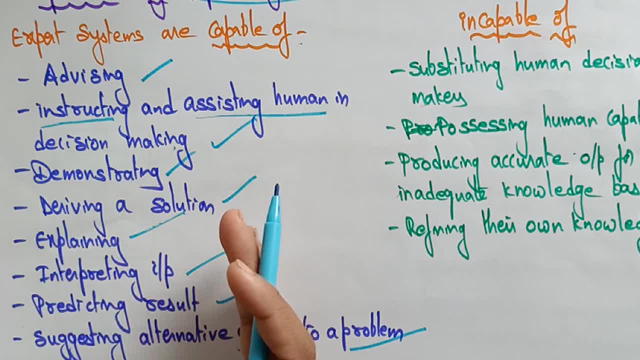 options. no, you can go in this way. no, it you can go at another way so that you you will get uh. there is a less traffic there. so it is going to uh suggest the options to a problem, so it is going to suggest the options to uh reaching a destination also. so these are all the uh expert systems that 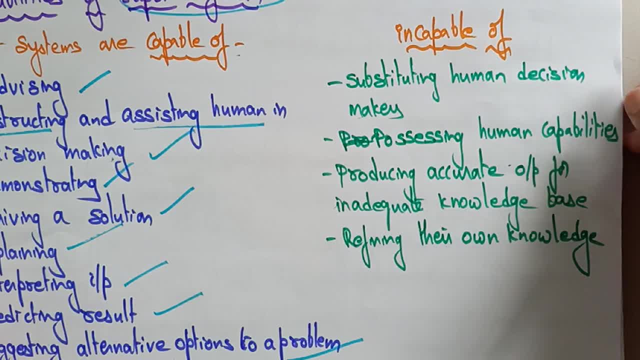 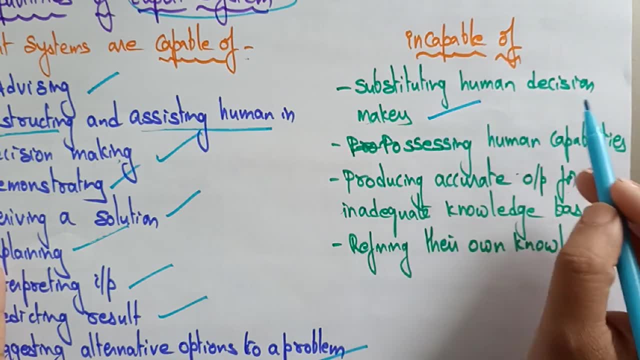 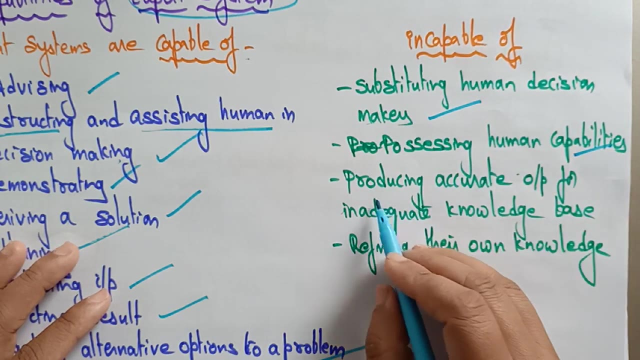 are capable of? and what are the expert systems incapable of? incapable of means? substituting human decision makers. substituting human decision makers that expert system cannot do. possessing human capabilities, producing accurate output for inadequate knowledge base. so, without the adequate knowledge, the expert system cannot give an exact output, the correct output. so producing accurate output for inadequate. 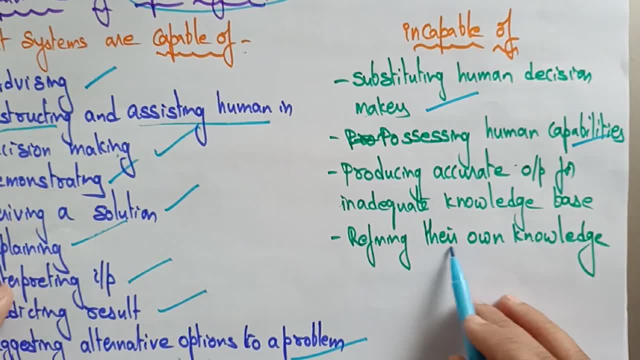 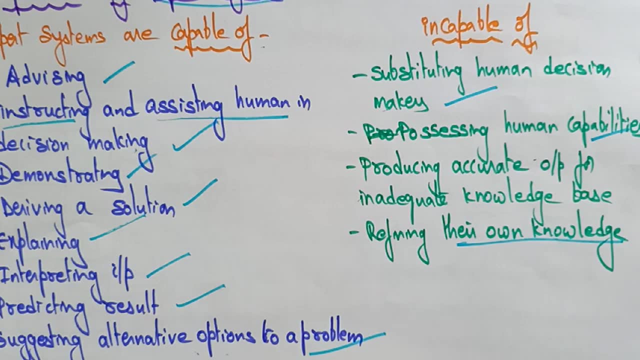 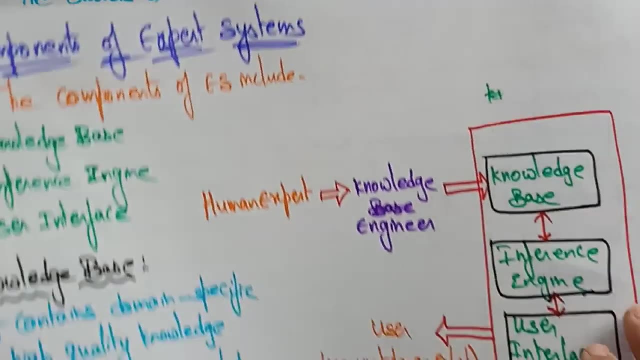 knowledge base is not, is incapable. refining their own knowledge is also not possible. okay, we are giving the instructions to the system so that it is working. this, whatever we are giving that, it is working, but refining their own knowledge is incapable. it can't do that. okay, so now let's. 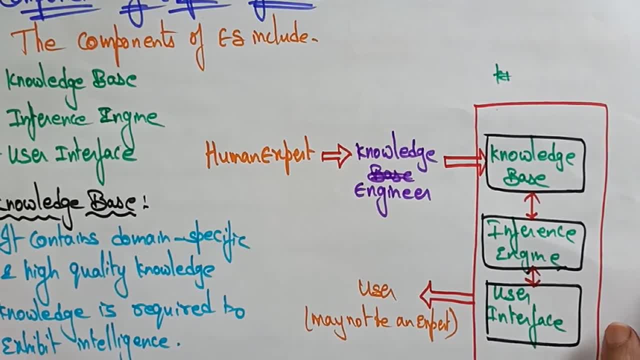 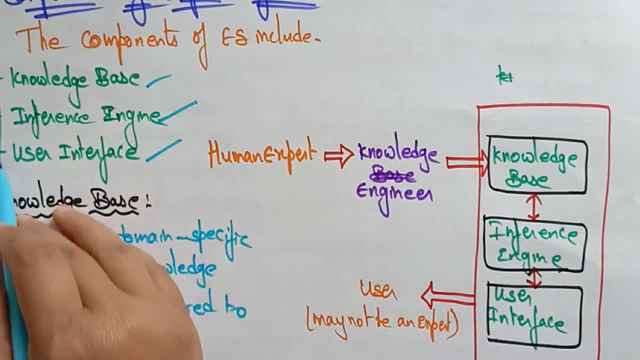 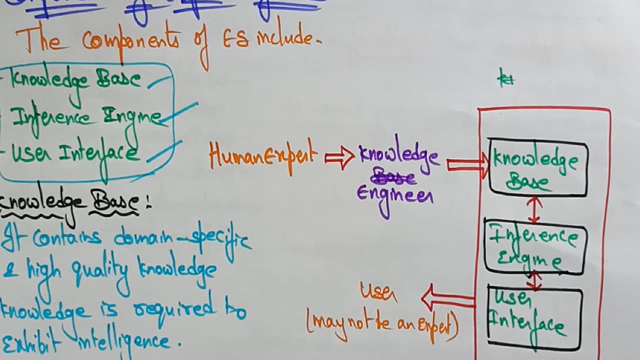 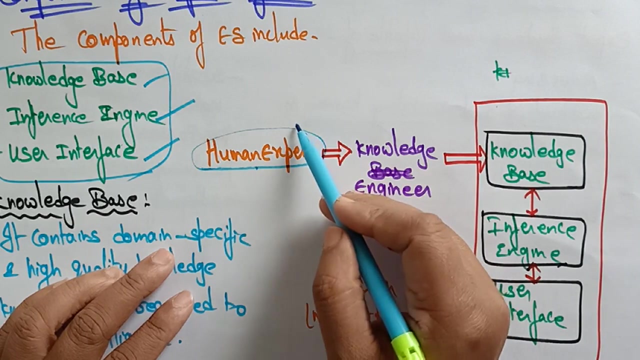 see the components of the expert system. the components of expert system includes knowledge base, inference engine, user interface. so these are the three basic components of the expert system. it is knowledge base. is there inference engine? is there user interface? so see here in the diagram. so this is an human expert. is there a person? the human expert is having the 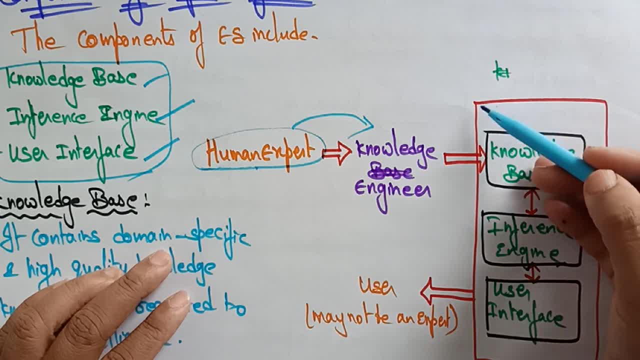 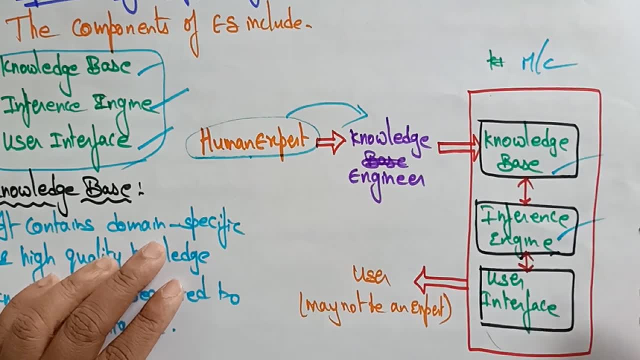 knowledge engineer. okay, with the help of the knowledge engineering, he going to design a machine, okay, a machine consisting of a machine which is a machine, which is a machine, which is a type of knowledge base inference engine, and that after that it has to communicate with the user, user. 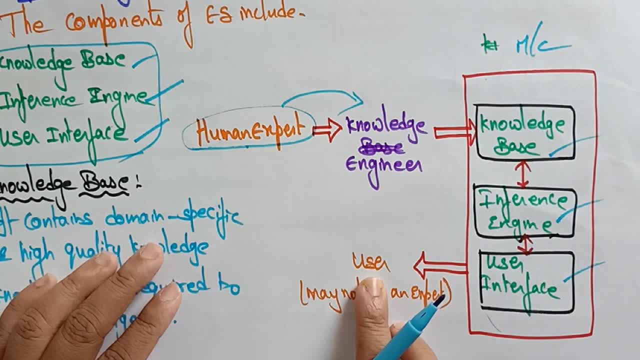 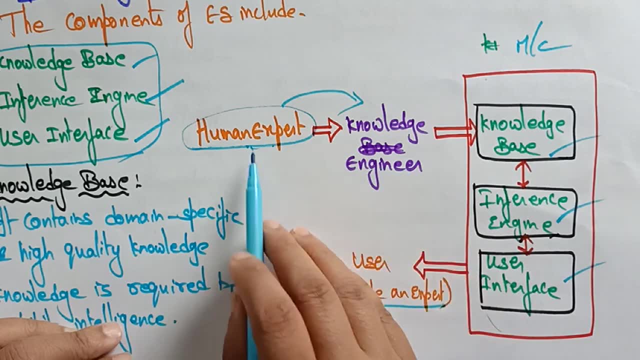 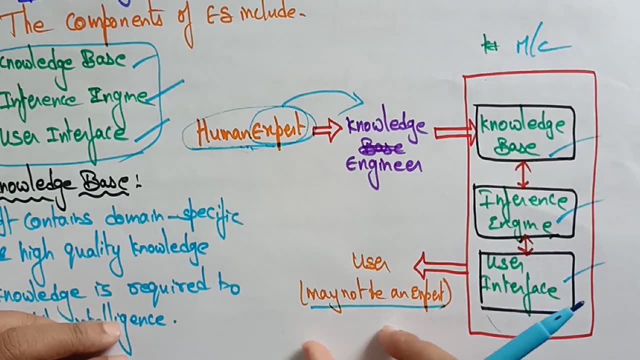 interface will be there, so then the user is able to see the output of what the machine is providing. so it's, the user may not be expert, but the human should be an expert, the person who implementing the machine, he should be an expert, he is a knowledge engineering, the user who is watching. 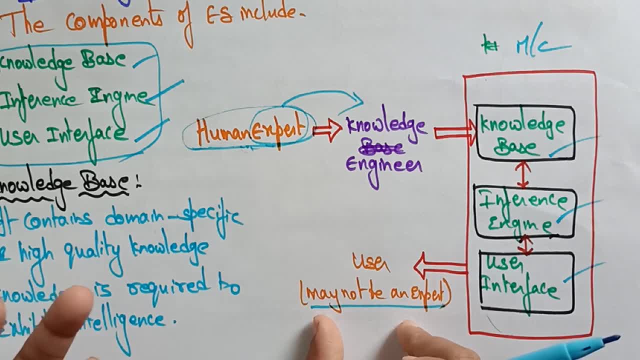 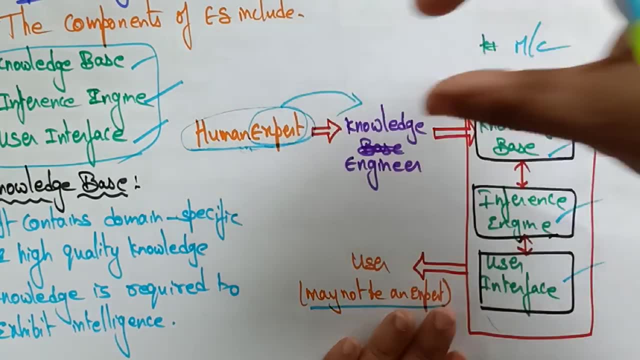 that and he who is using that machine may not be expert. okay, so the user who is watching that machine, so he, he, he doesn't bother about what is there inside, but here the human expert, he has to know what is there in the machine because he is a person who is inserting the knowledge in the machine. 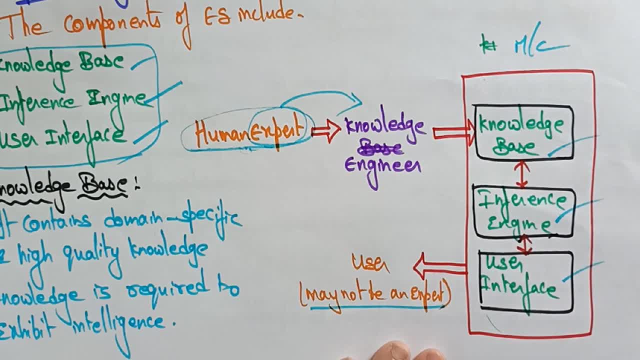 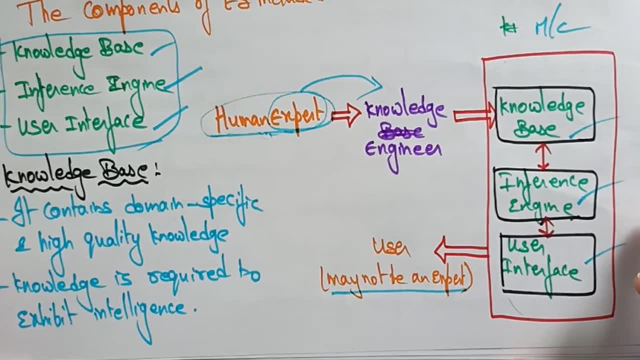 so in the machine knowledge base is there inference engine is there and user interface. so let's see one by one in in clearly: what is the knowledge base, what is inference engine and user interface? okay, knowledge base. it contains a domain specific and high quality knowledge. so, whatever the 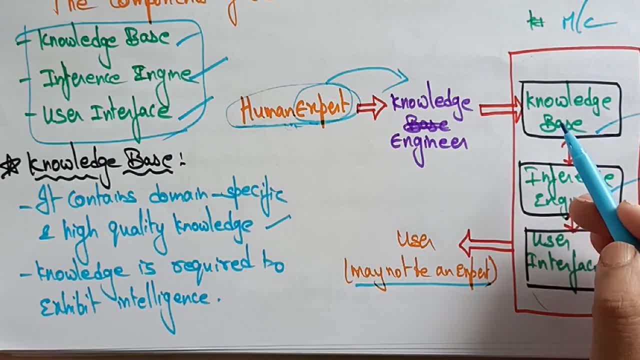 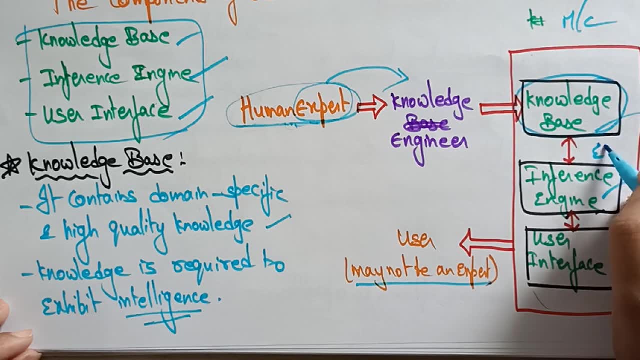 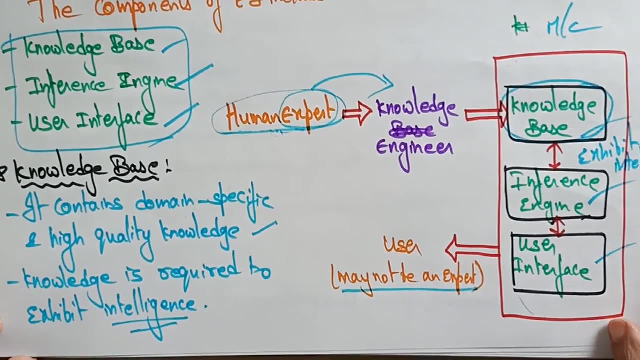 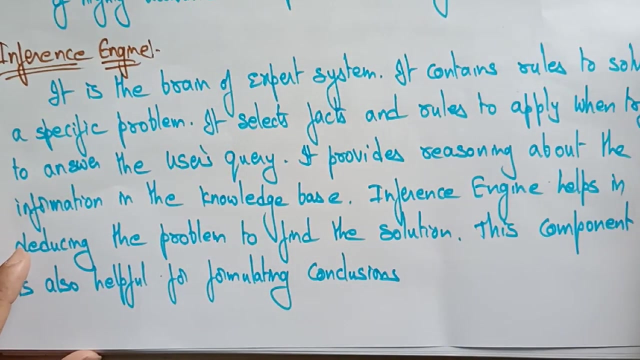 knowledge base that we are using. it has a domain specific and high quality knowledge, and knowledge is required to exhibit intelligence. so, whatever the knowledge that it is having, it is going to exhibit intelligence. it is exhibiting the intelligence so that the inference engine can work according to that uh intelligence and, next step, the success of any uh expert system. 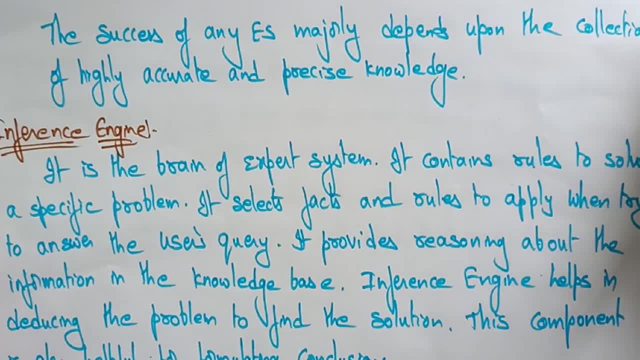 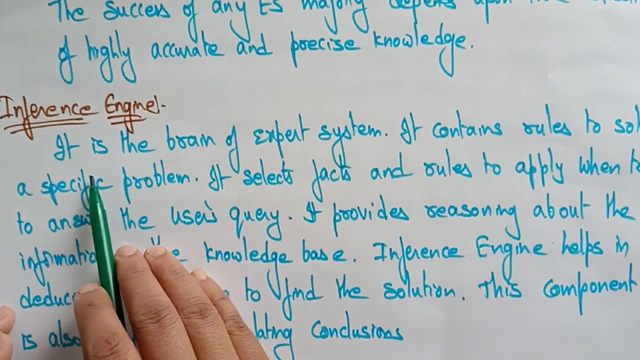 majorly depends upon the selection of highly accurate and precise knowledge. so that is about the knowledge base. so next is the inference engine. so what is this inference engine? so it is actually in between the knowledge base and the user interface. this inference engine, uh, is the brain of the expert system. we call it as a 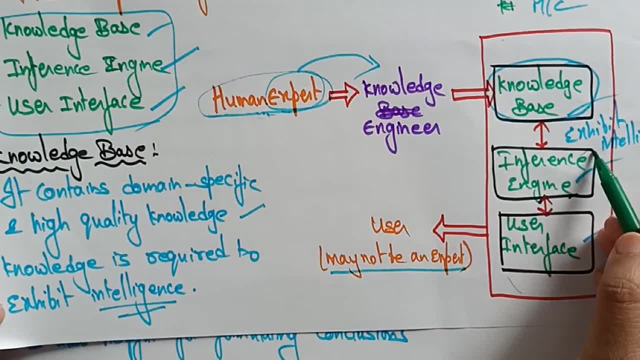 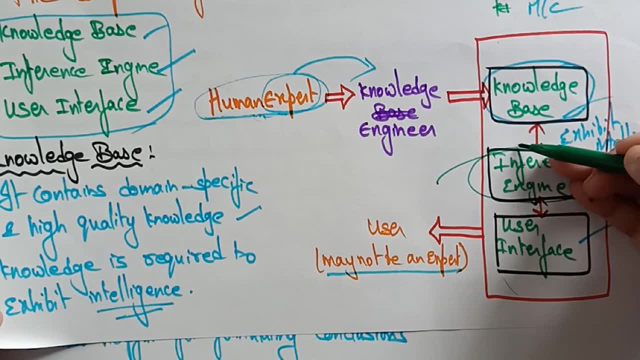 brain of expert system. so in the diagram you can see where the everything will be work in this inference engine. the knowledge base is just giving an exhibits the intelligence to the inference engine. the inference engine performs the operation and uh gives to the user interface. then the user inter with the help of user interface we are 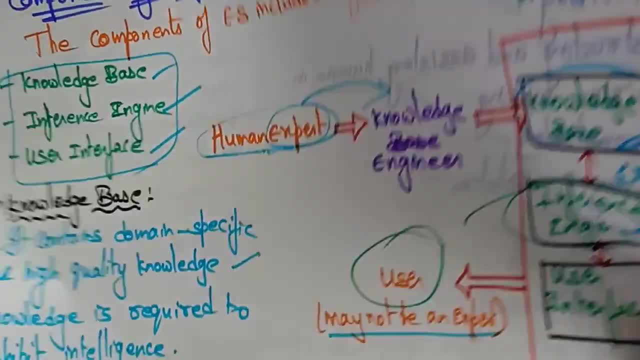 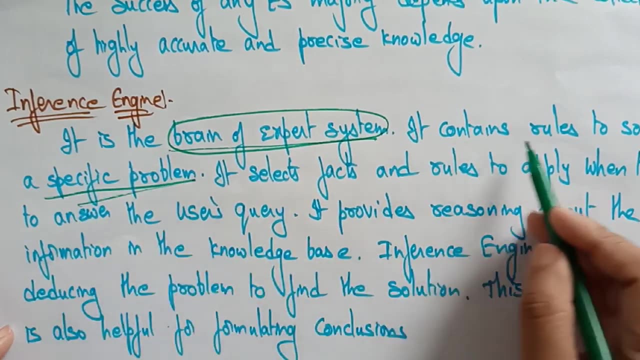 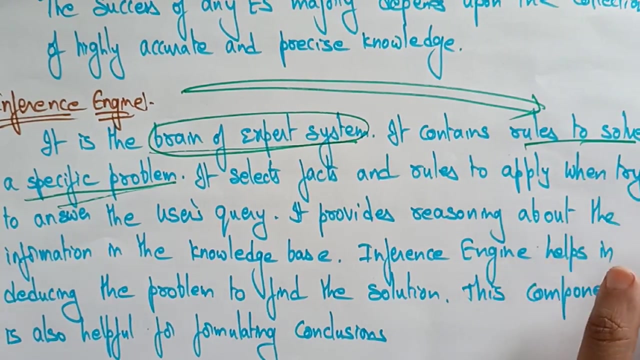 the user can able to use that machine. so inference engine is the brain of expert systems. it contains rules to solve the specific problem. so in the inference engine you are having some rules. okay that rules are used to solve the specific problems. it selects the facts and rules to apply when. 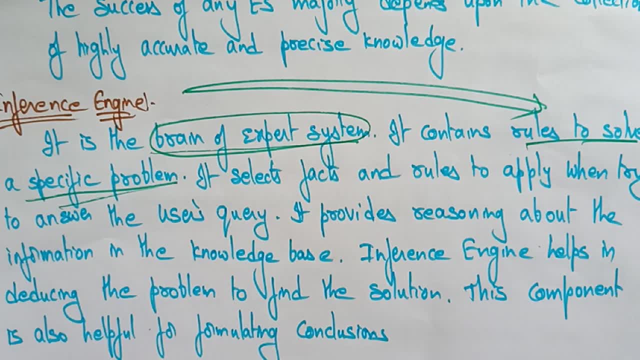 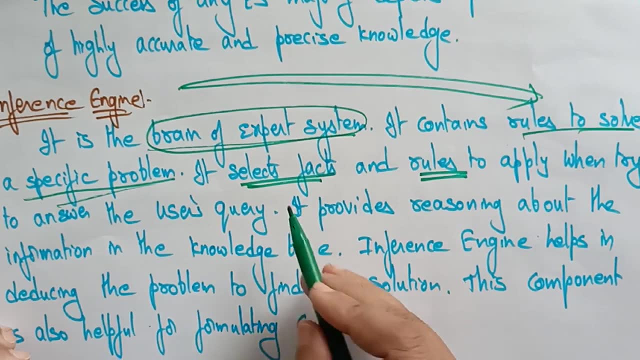 trying to answer the user queries. so whenever, when the user is trying to answer the user queries, when this inference will- uh, injury will be used, it is going to select the facts and whatever the rules that are it contains, with the help of the facts and rules to apply when trying to answer user queries. 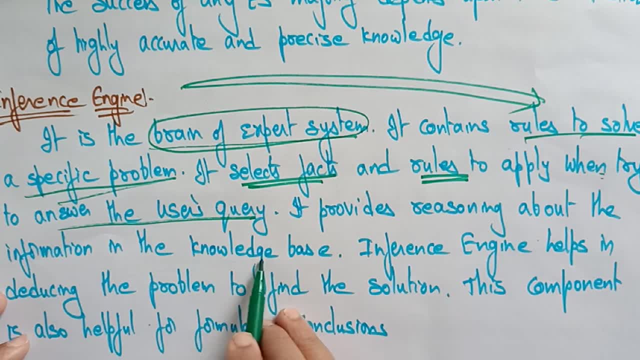 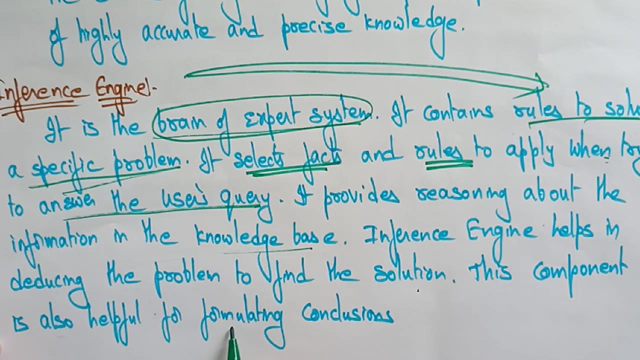 and this inference engine provides a reasoning about the information in the knowledge base. so with the help of the knowledge base only it is going to solve the problem. it going to answer the user queries. inference engines helps in deducing the problem to find the solution, and this component is also useful for formulating the conclusions also. so everything, uh, we are. 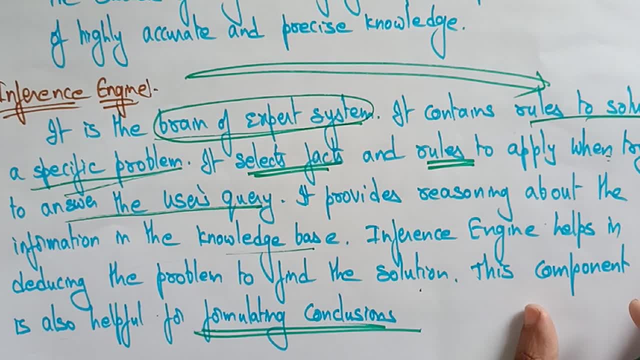 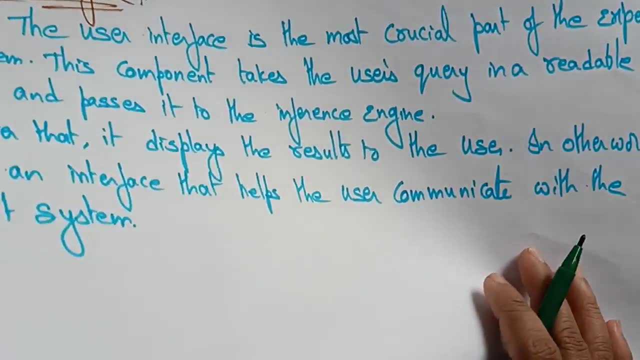 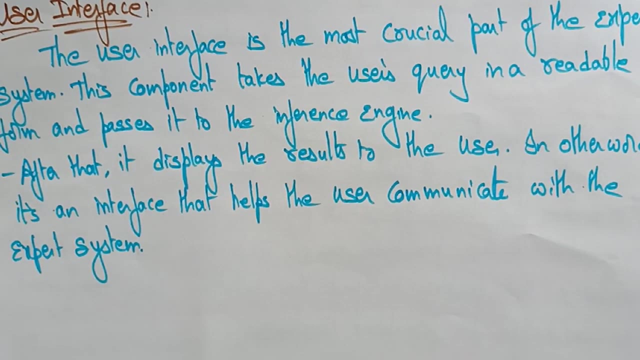 performing in inference engine by taking the input from the knowledge base. so that's why we call it as a brain of expert system. and the last component in this user interface is sorry. expert system is the user interface, so it's access and influence between the user and the influence. 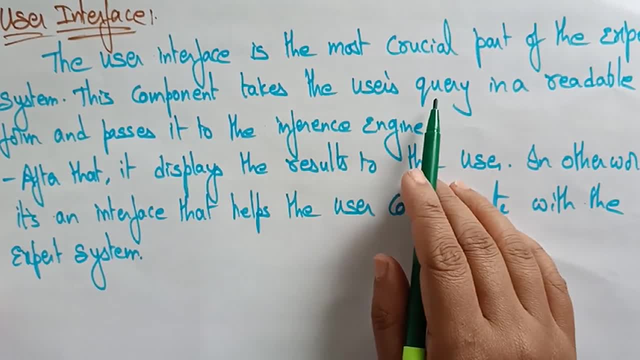 inference engine. the user interface is the most crucial part of inference, so it acts as an inputs between the user and the influence influence engine. the user interface is a most crucial part of this experience. you are not going to be able to solve the problem in the knowledge base. 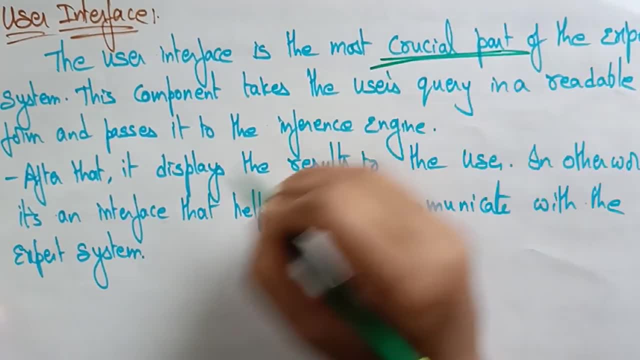 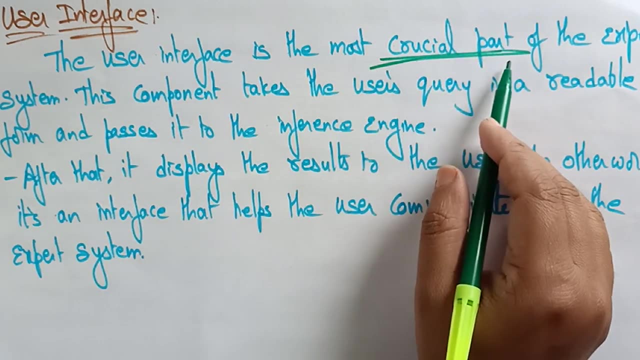 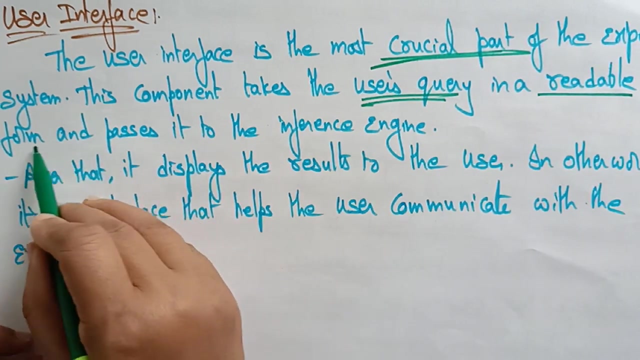 the expert system. oh, it's a very crucial part, okay, because it is going to communicate with the user. so the user interface is a most crucial, crucial part of the expert system. this component takes the user's query in a readable form and passes to the interface engine. so i am the user, okay. 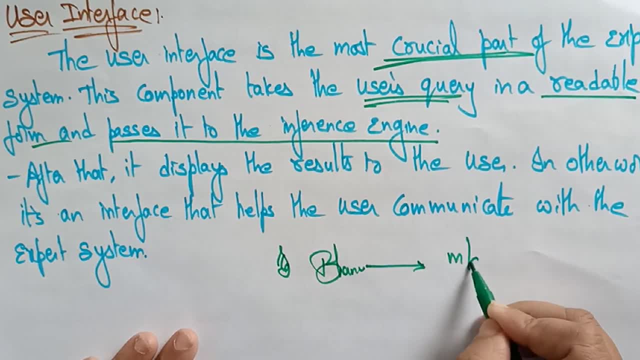 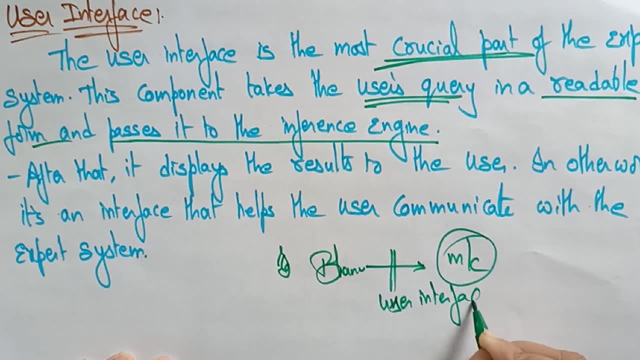 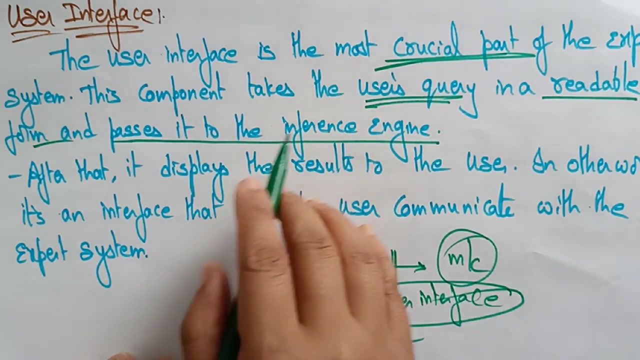 i am the user, i am interacting with the machine. how i can interact with the machine with the help of the user interface, user interface. what this user interface is doing, it is taking the query from the user in a readable manner, in a readable form, and passes to the inference engine. 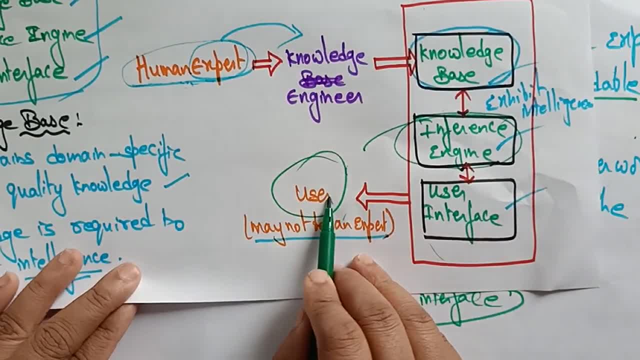 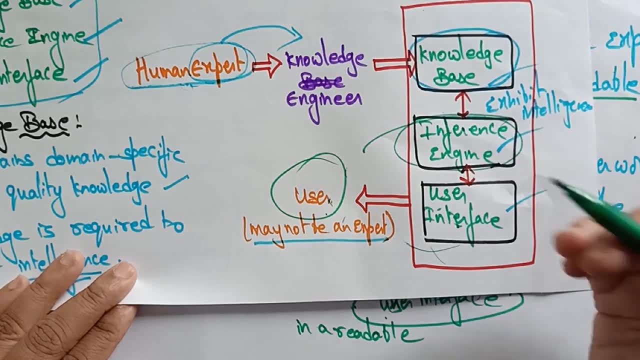 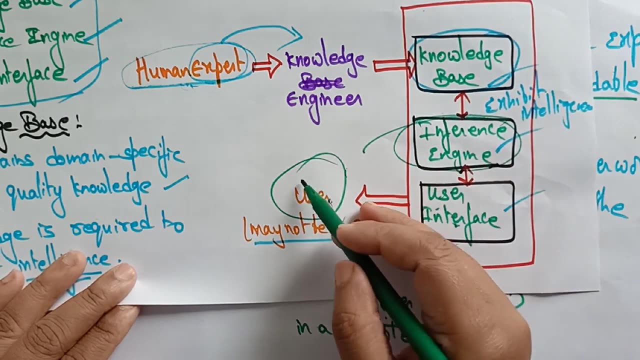 so, whatever the engine that is present, okay, it's just taking the input query from users and converting that in a readable format to the inference engine. because the inference engine cannot understand the english language, it has to be converted. okay, so here everything will be in between like this: so, uh, user in user, user interface and interface engineering is performing. 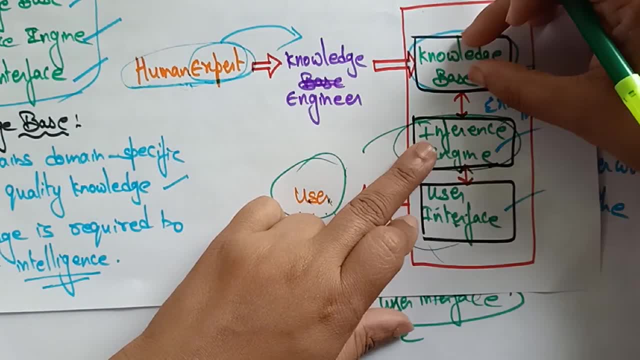 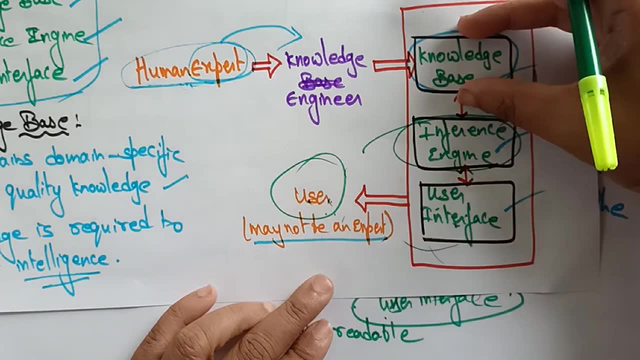 based on the knowledge base given by the expert system, taking the knowledge from the knowledge base and performs the operation and again sends the result to the user. okay, so this part is a constant. okay, this part is a constant. so here the operations are performing in between this. 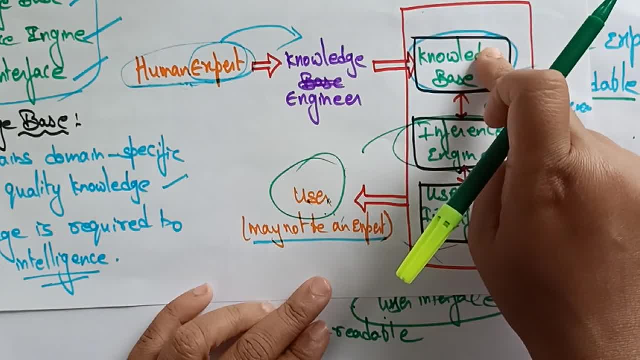 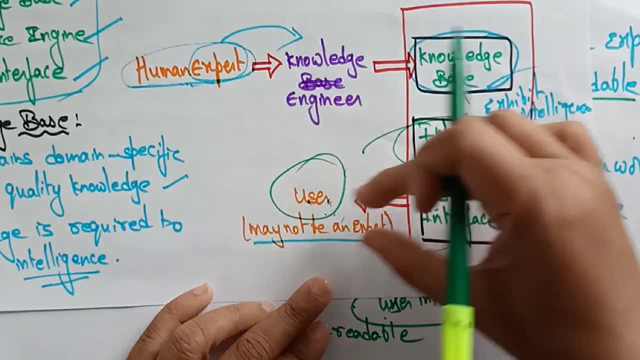 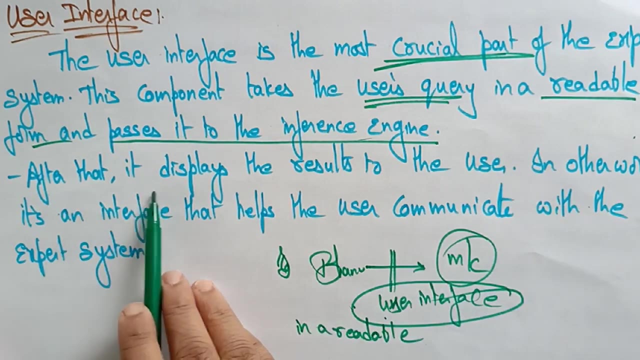 in between this, The knowledge base is given by the human expert and it will be the constant. With the help of the knowledge base, only the inference engineering is performing the operations according to the user queries. I think you get it. Okay, let's see. After that, it displays the 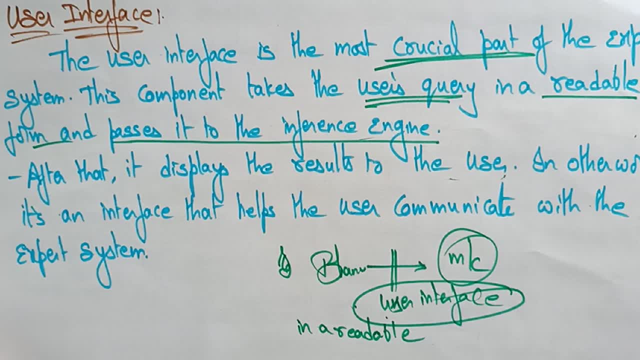 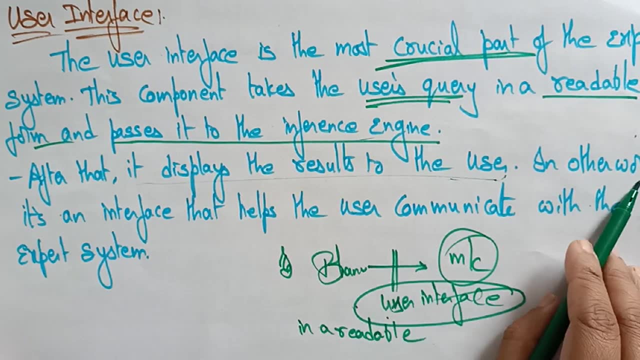 results to the user. Okay, whatever the information it is taking from the knowledge base and the inference engineering sends the result to the user interface and it displays the results to the user. In other words, it's an interface that helps the user communicate with the expert system. So 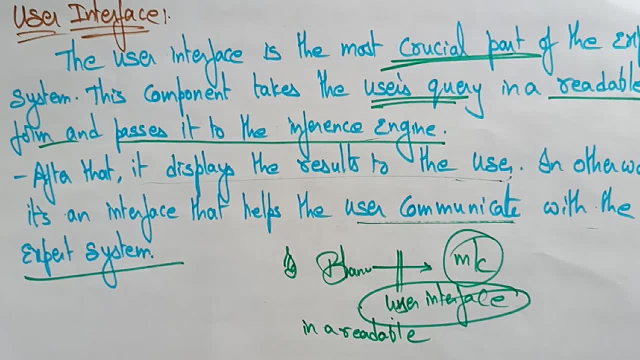 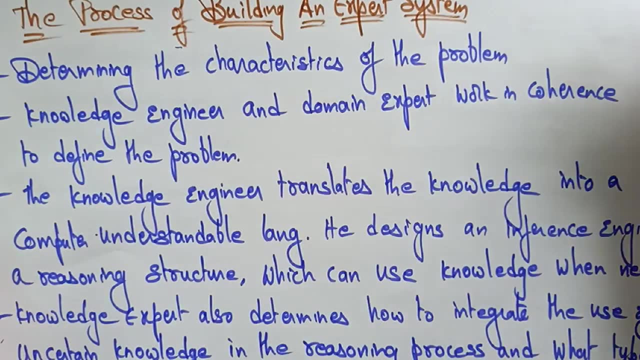 just user interface is acting as an interface between the user communication and the expert system. So these are all the components of the expert system. Let's see the process of building an expert system: How you are going to build an expert system. Okay. 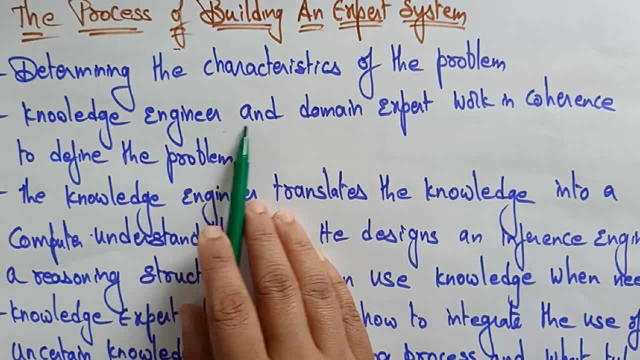 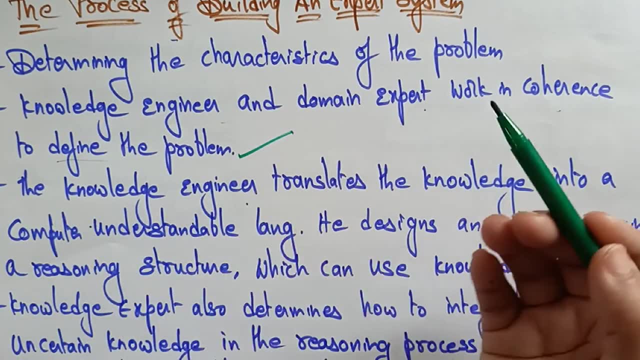 Determining the characteristics of the problem. The knowledge engineering and the domain experts works in the coherence To define the problem. Next, the knowledge engineering. whatever the knowledge engineering is there, the person is going to translate the knowledge into a computer understandable language. 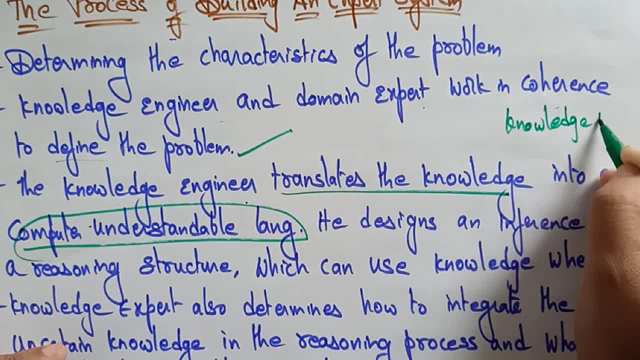 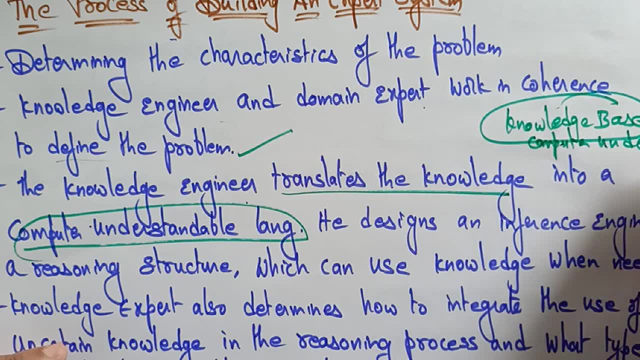 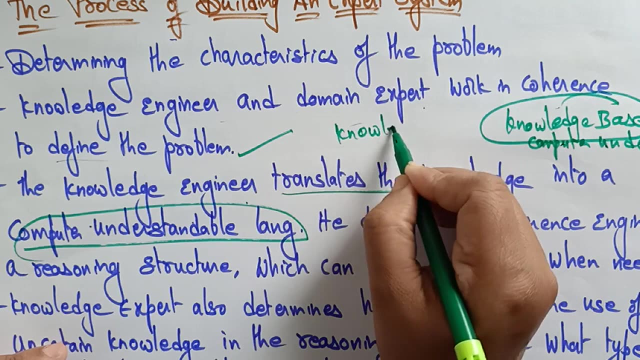 So, whatever the knowledge base is there, okay, in the knowledge base everything should be in the form of computer understandable way, So that the interface engine can take this information from the knowledge base. So here the knowledge engineering, whatever the knowledge engineering.